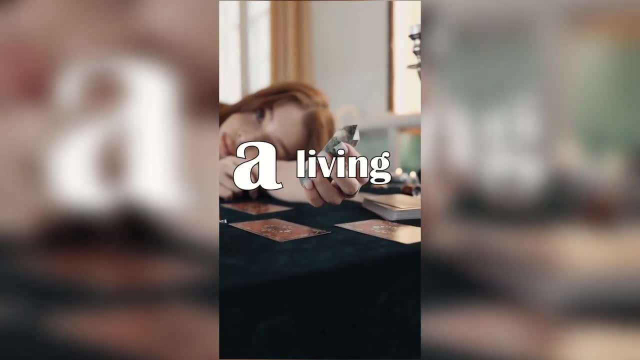 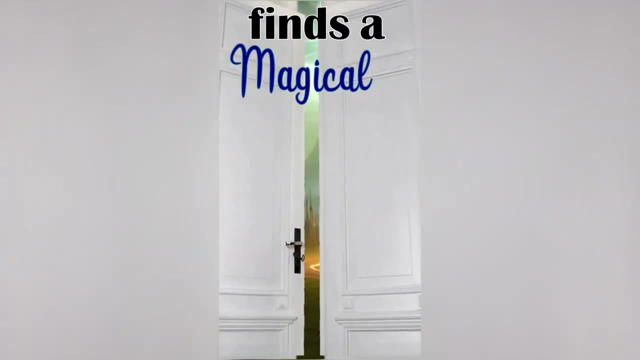 but isn't sure if they believe it. Your character makes a living faking psychic powers. One morning they wake up with real ones. Write a story about someone who finds a magical portal in their home. Write about a character who wakes up in their past life. 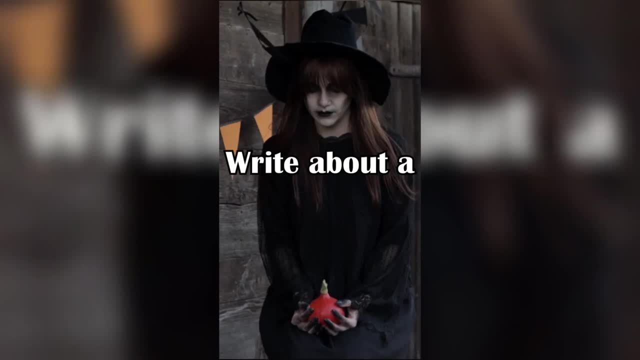 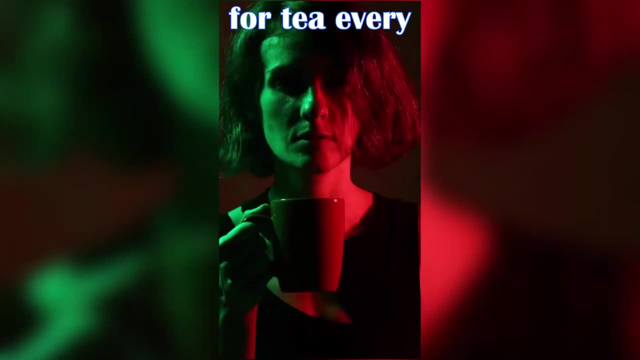 or as a future reincarnation of themselves. Write about a mischievous pixie or trickster, god. Write about a person who meets the ghost of an old friend for tea. every so often, As you're paying for your groceries, you mention to the clerk. 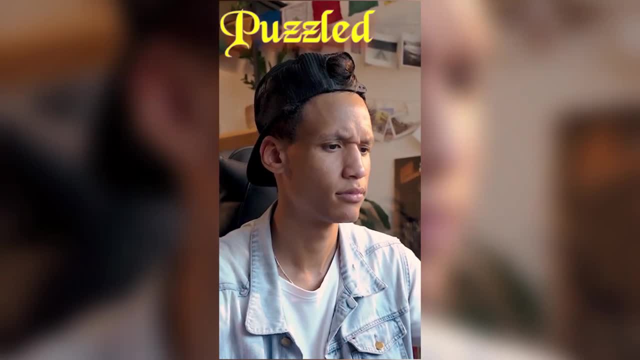 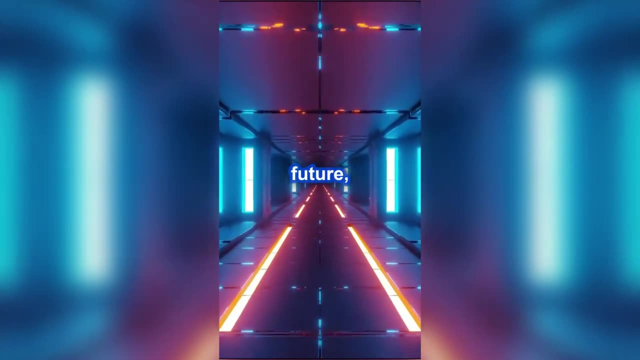 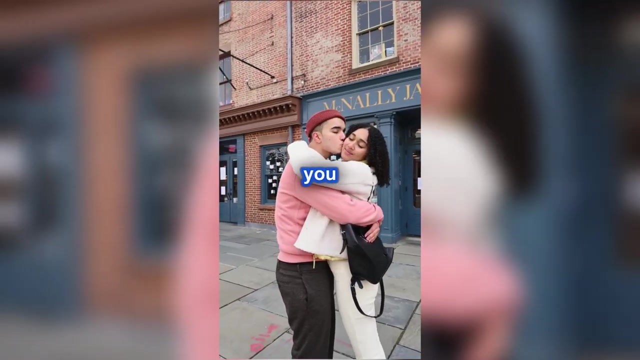 there's a mess in aisle 24.. They give you a puzzled look and reply: there is no aisle 24.. In the future, romantic attraction is literal. Each person is fitted with an electromagnetic bracelet which they claim will pull you to your soulmate. It's the day they turn on the magnets. 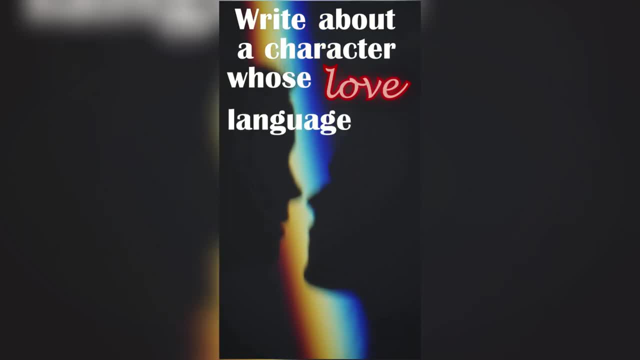 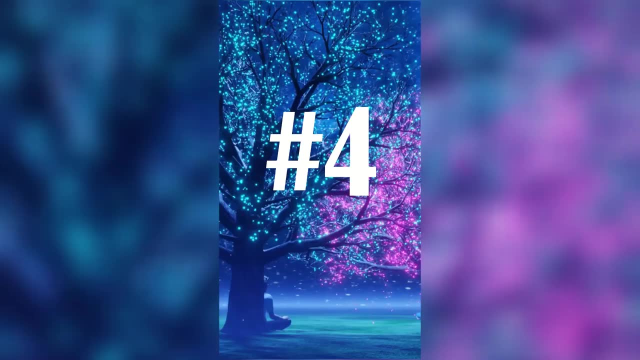 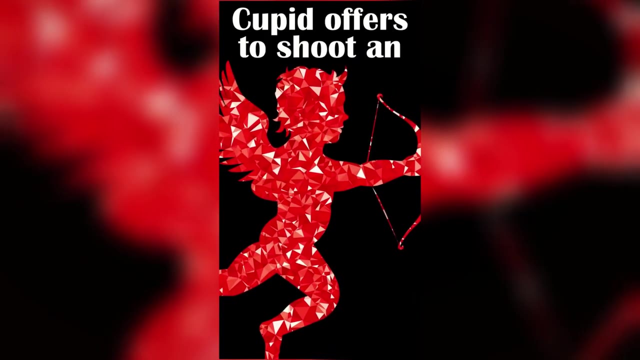 and you're waiting. Write about a character whose love language is making food for others. End your story with a kiss at midnight. Write about two solo travelers who keep bumping into each other in the most unexpected of places. Cupid offers to shoot an arrow into the person you love, but he warns you that if the person 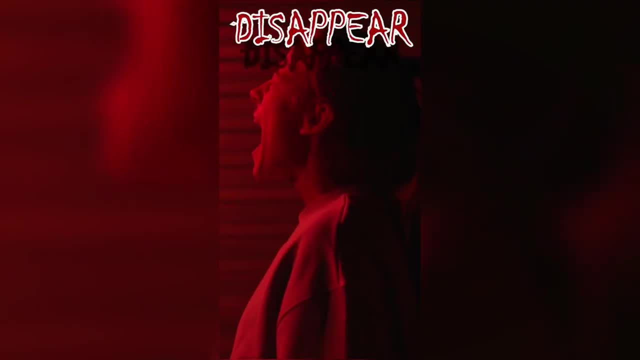 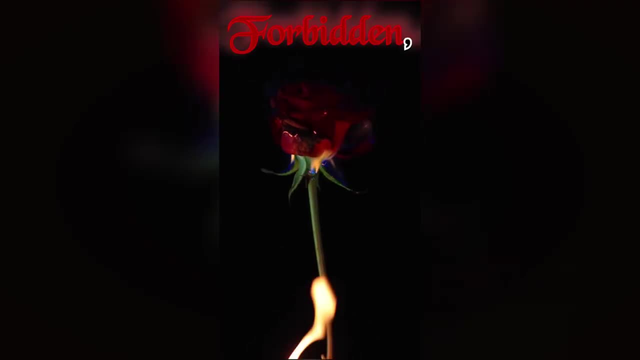 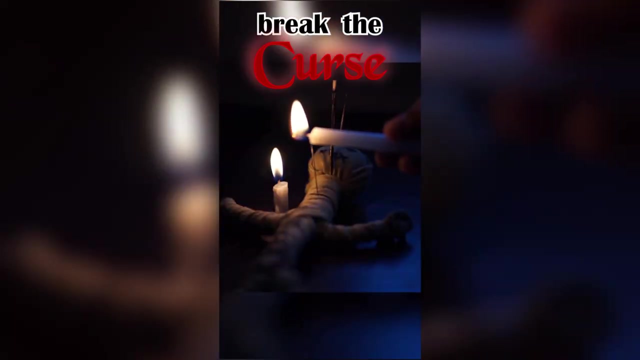 already has a pre-existing affection towards you, it will disappear when the arrow strikes. She was a mermaid and he was a prince. Their love was forbidden, but they couldn't resist each other. She was a powerful witch, but he was the only one who could break the curse. 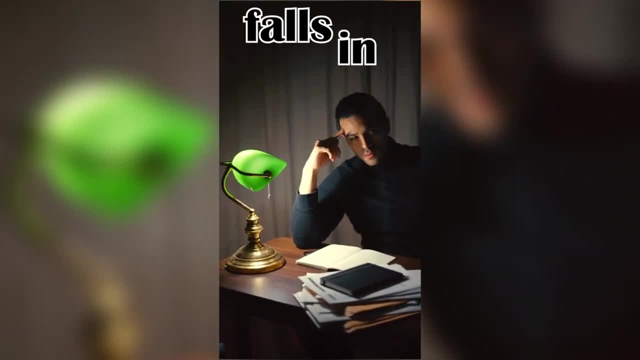 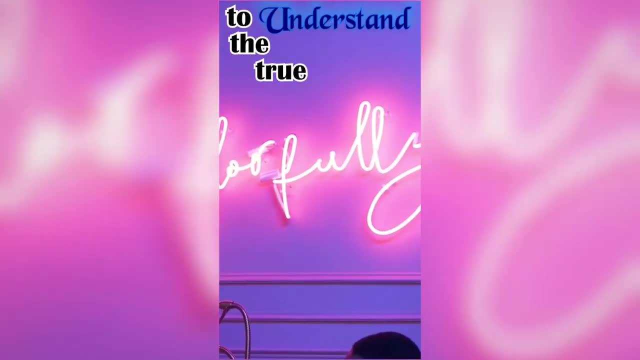 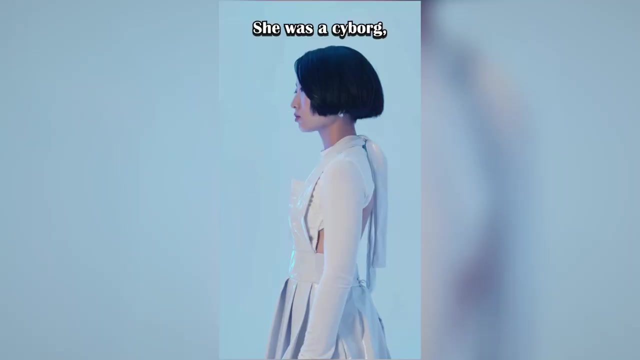 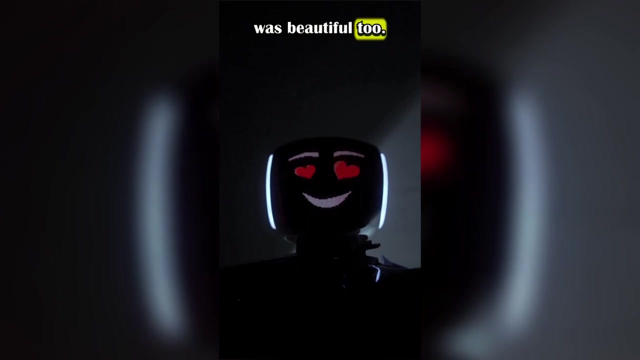 that haunted her. An aspiring writer falls in love with a reclusive, enigmatic author, but must uncover the secrets of his past to understand the true nature of their relationship. Write about a character who risks everything to pursue their heart's desire. She was a cyborg programmed to be perfect, but he showed her that imperfection was beautiful too. 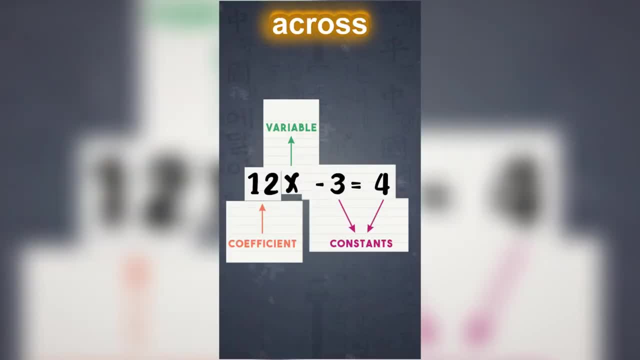 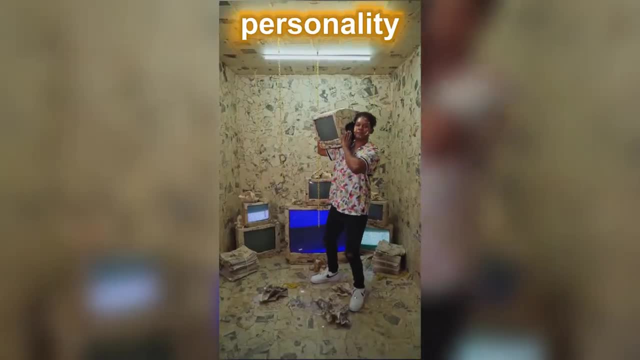 There's only one constant across the multiverse: Adam Sandler. No matter how joyous or bleak a universe is, he's always there, alive and well, with the same personality and comedy. No humans in a universe Still there. It can get ridiculous. 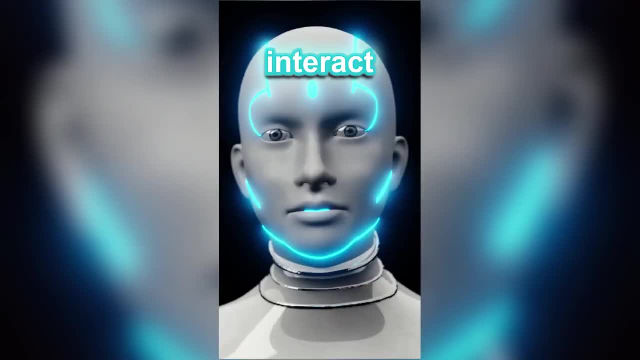 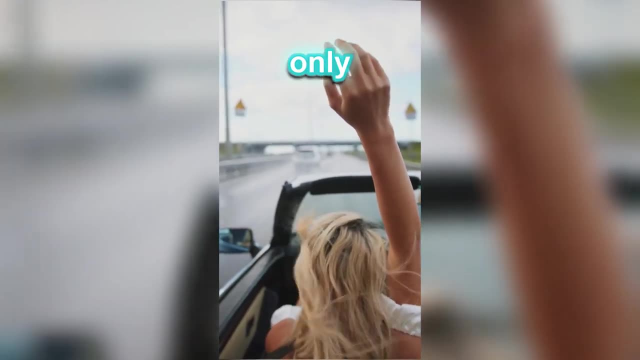 In a dystopian future, all machines use voice to interact with humans seamlessly, With no need to read or write. mankind lost these skills. People only lived for the moment. But all that changed when a machine was able to read and write. A machine that could read and write. A machine that. 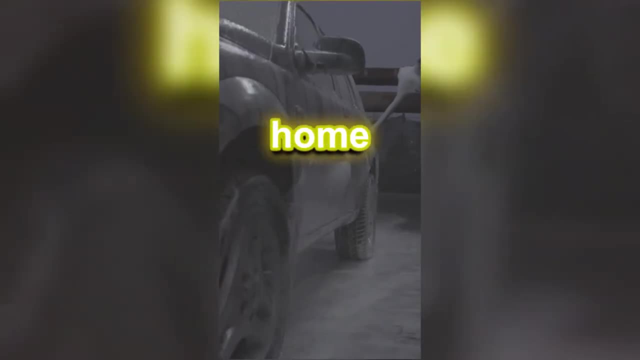 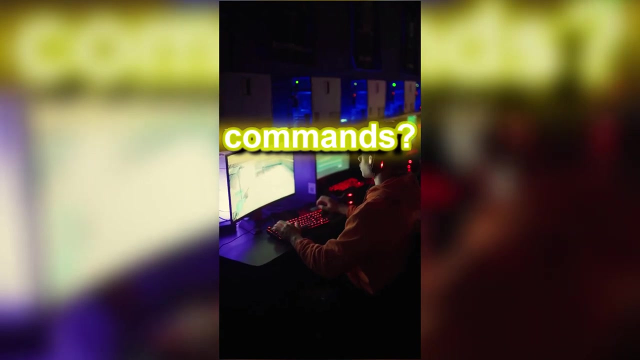 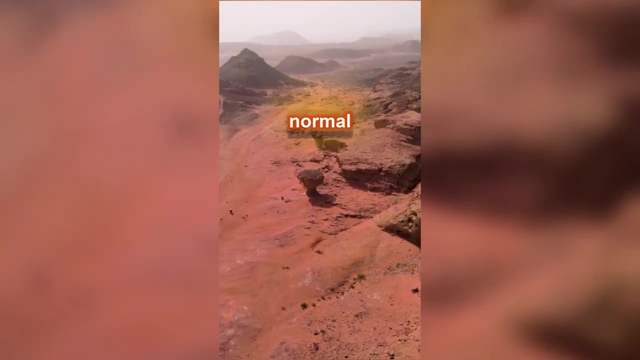 taught a girl to read and write. You stay home from work one day feeling somewhat ill, only to hear a voice in your head. Why isn't he obeying my commands? This game is bugged. NASA engineers monitor the Curiosity rover's actions. All seems normal until the 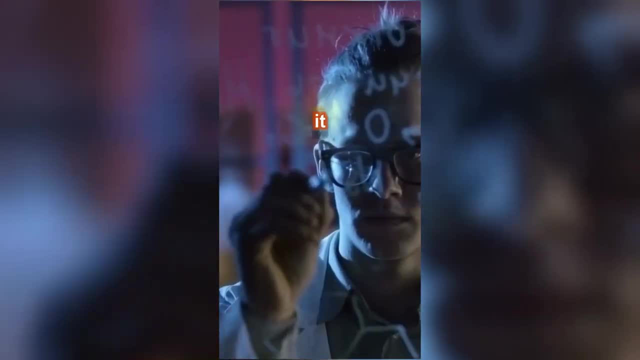 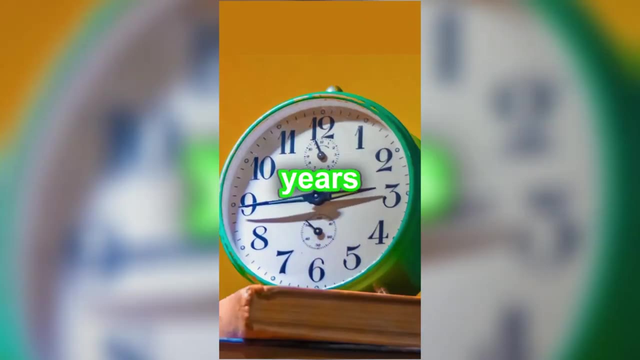 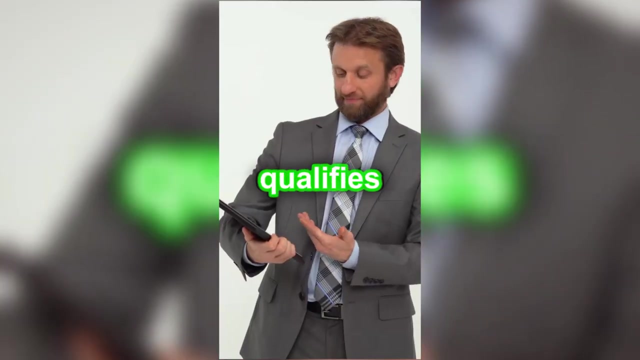 robot suddenly changes its course. The scientists attempt to correct it over and over until they suddenly receive a transmission from the rover. We'll save Oppie Ten years from now. scientists figure out how to stop human aging and extend life indefinitely. But every time someone qualifies. 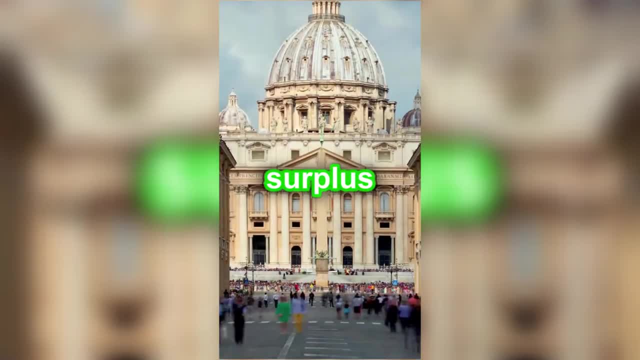 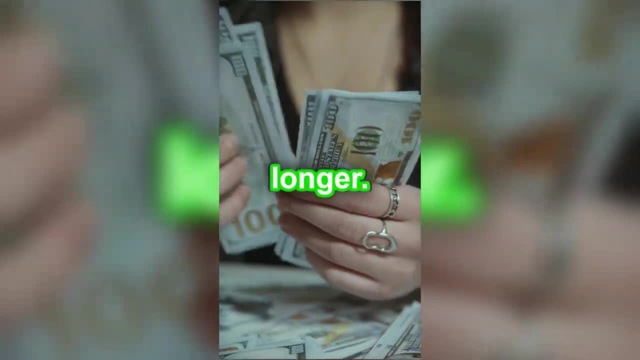 for that boost. someone else must die to keep the surplus population in check. It's all humane because the descendants of the person killed is financially supported by the person who gets to live longer. Now you've just got a letter in the mail saying you're the one who has to die. 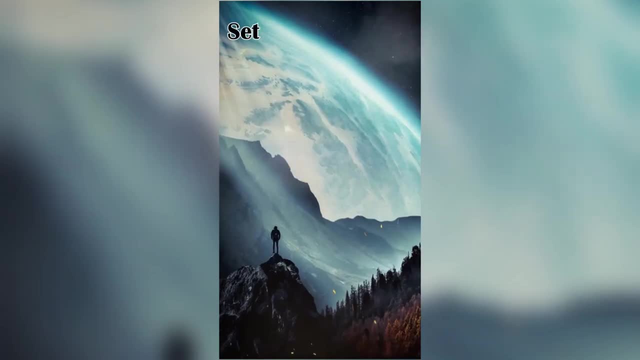 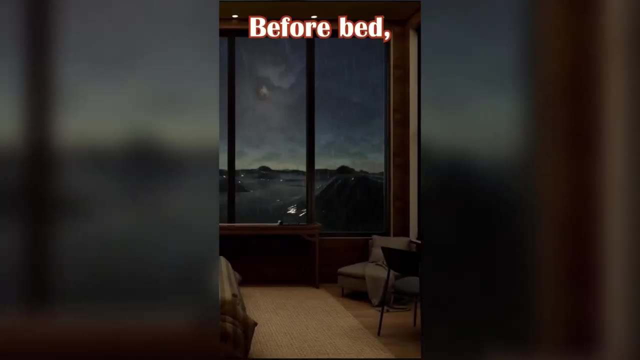 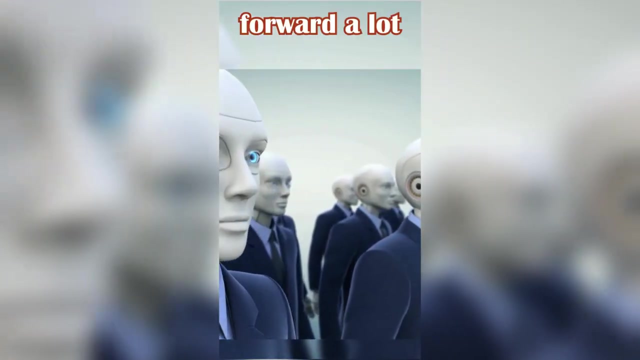 Set your story in a nameless world. Set your story in a world where the currency isn't money, or at least not money as we understand it. Before bed, you put your clock ahead one hour for daylight savings time. When you wake up, you realize you've gone forward a lot more than one hour. 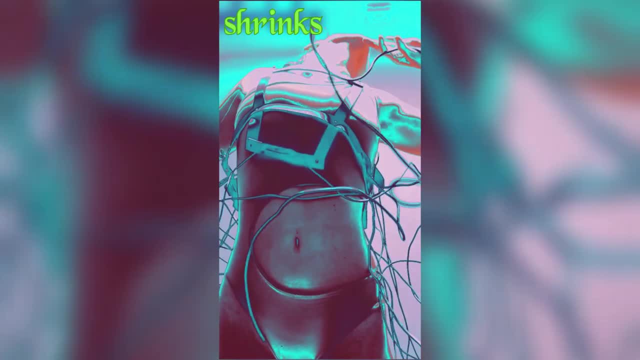 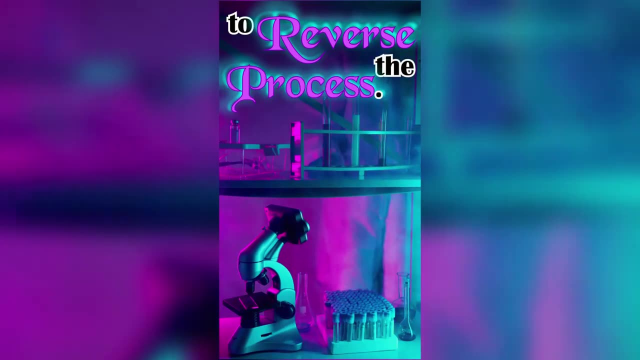 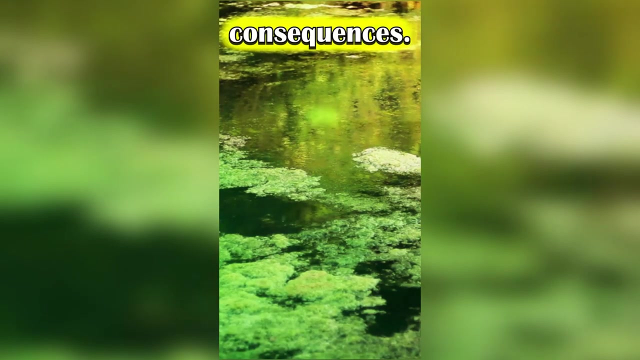 After a failed experiment, a scientist accidentally shrinks herself down to the size of a bug and must navigate her way through her lab to find a way to reverse the process. Write a story about a scientist who creates a new form of life, with disastrous consequences. 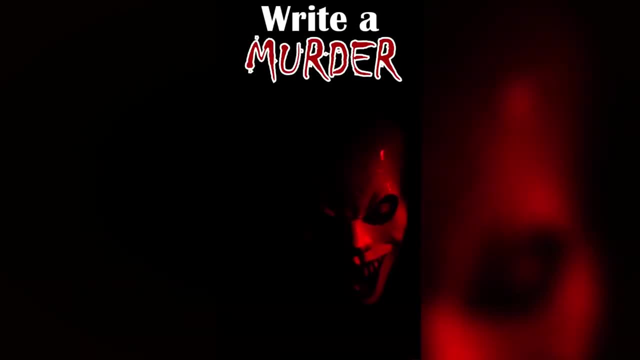 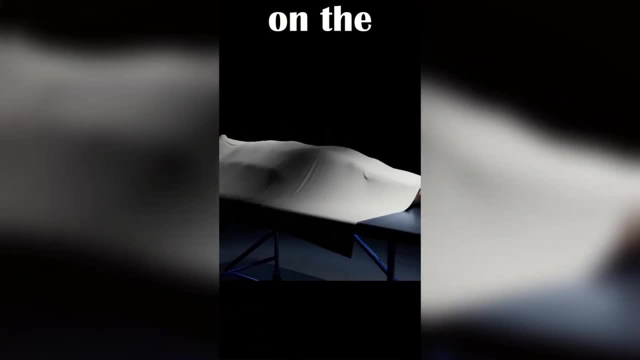 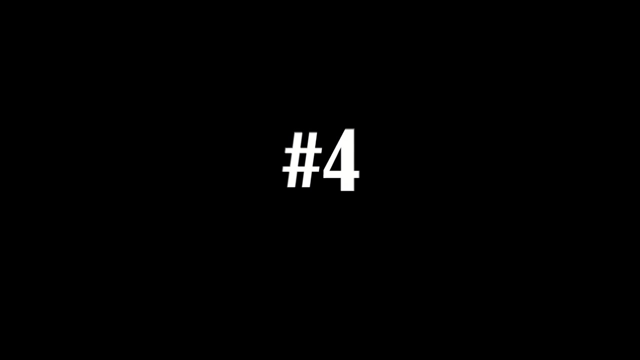 Write a murder mystery where the murder weapon is the knife used to carve a pumpkin. Write a story that hinges on the outcome of a coin flip. Big Brother is real and it's you. Write about a zombie apocalypse, but from the perspective of a terrified zombie. 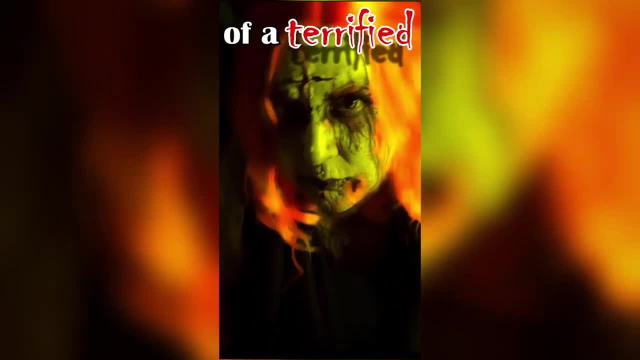 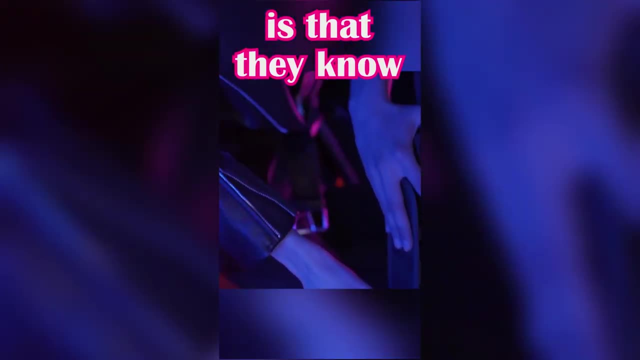 Two people become internet friends. What neither realizes is that they know each other in real life. The two become friends, but they don't know each other in real life. The two become friends, but they don't know each other in real life. 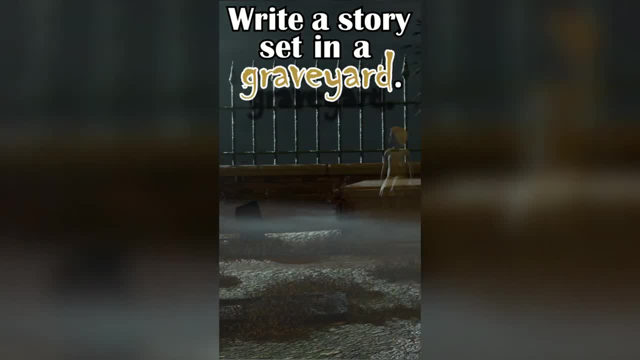 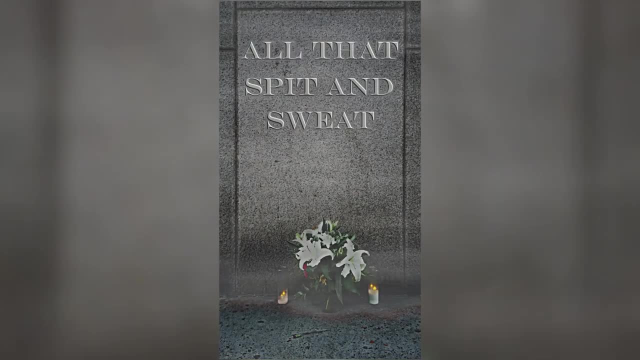 The two become friends, but they don't know each other in real life. Write a story set in a graveyard. Include a blue-veined hand, a serial killer and the phrase all that spit and sweat. She knew there was something off about her neighbor. 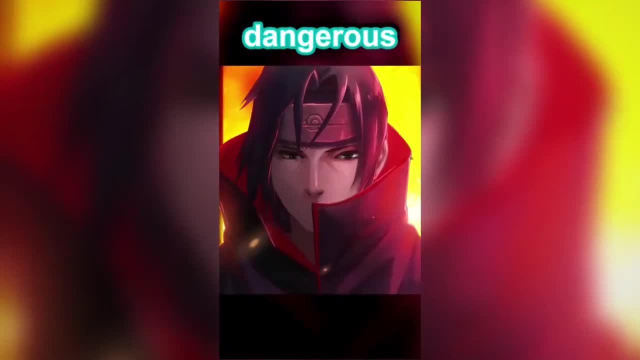 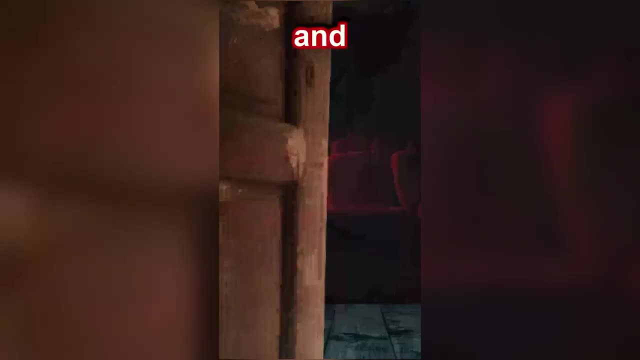 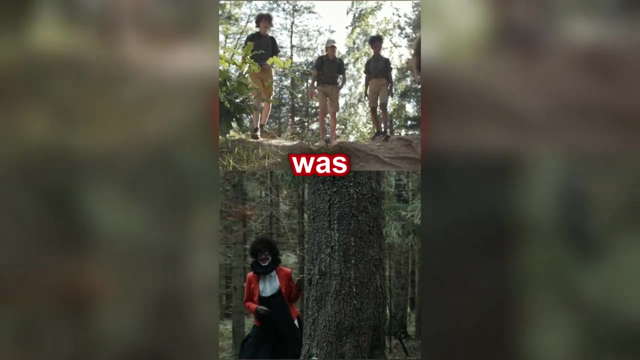 but she could never have imagined just how dangerous he was. A group of friends stumble upon a hidden room in an old mansion and uncover a dark and sinister secret about its past occupants. The summer camp was supposed to be a chance to make new friends. 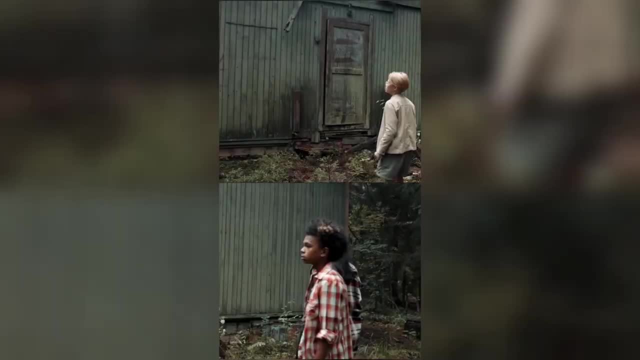 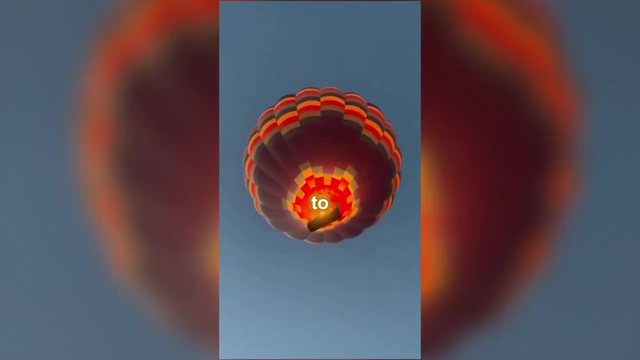 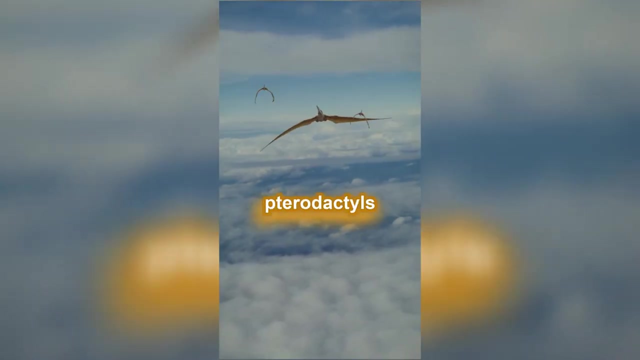 but it turned into a nightmare when they discovered the dark secrets hidden in the woods. A hot air balloon operator caters to folks who like a little thrill, which means she spends half of her time in the air shooting down pterodactyls before the customers get too scared. 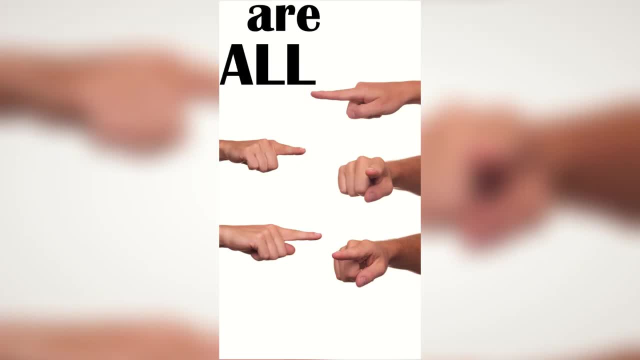 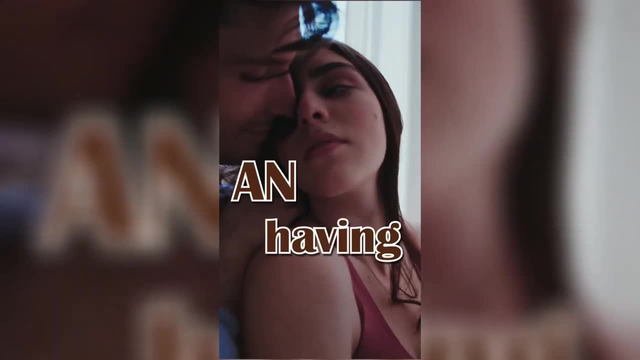 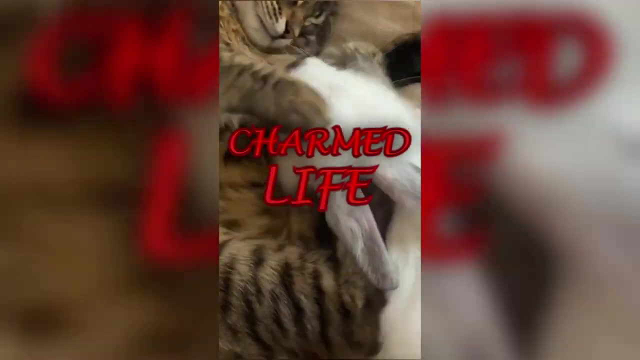 Write a story where a murder occurs and the suspects are all pointing the finger at one another. Start your story with a character telling their best friend that their spouse is having an affair, only for their friend to shoot the messenger. Write about a character who lives a seemingly charmed life. 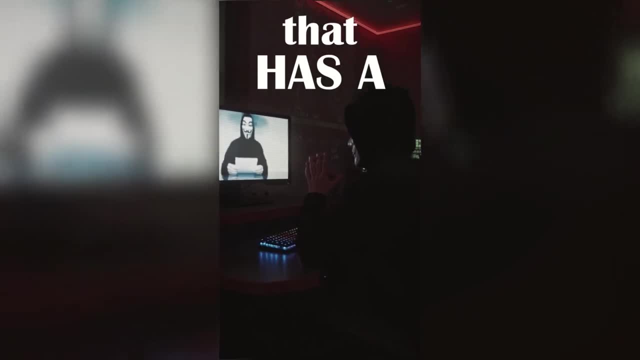 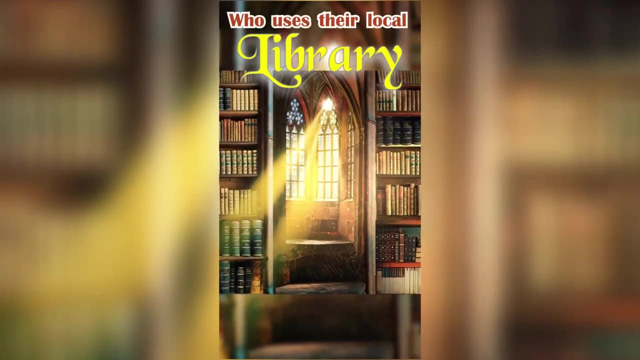 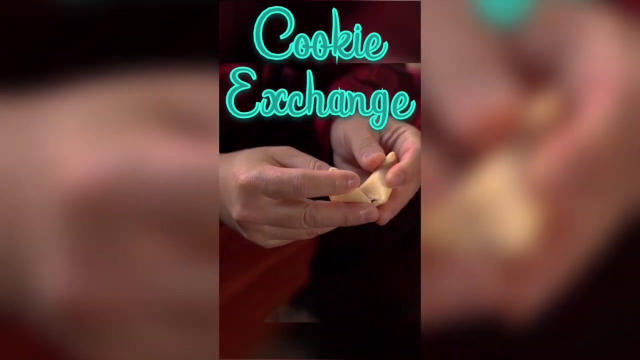 Start your story with someone sharing a secret that has a big impact on everyone. Write about a character on the hunt to solve a mystery who uses their local library or librarian as a source of information. Write about someone hosting a cookie exchange as a cover to hide the true reason for inviting one of their guests. 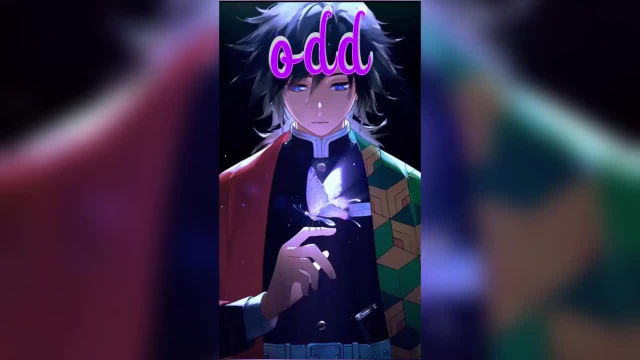 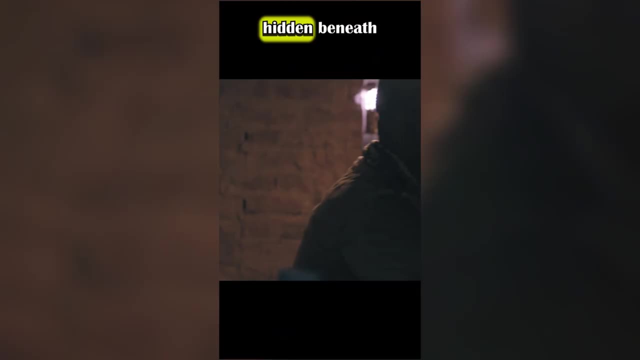 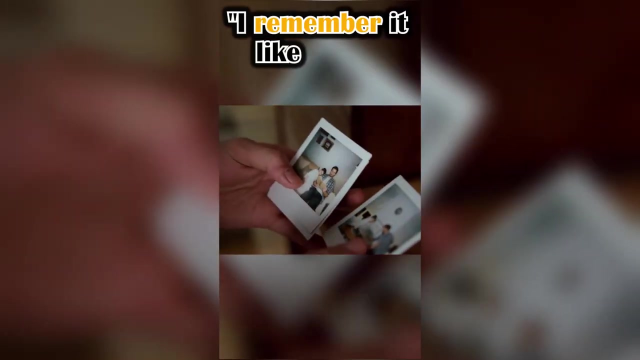 As you're taking down a painting, you notice something odd engraved on the back. The small town had always seemed idyllic until the secrets hidden beneath the surface began to emerge. Dialogue story prompt: I remember it like it was yesterday, but it couldn't have happened. 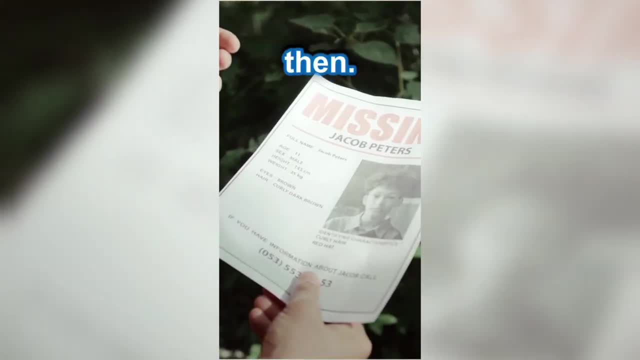 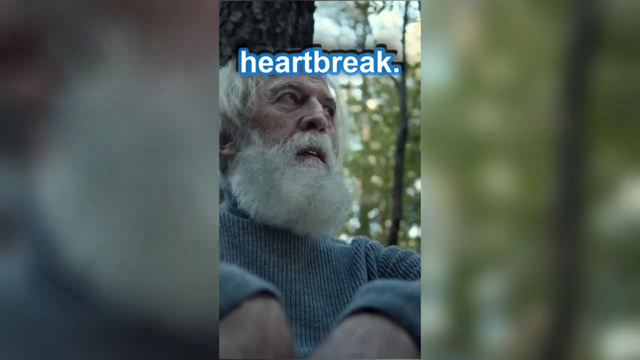 He went missing 12 years ago. He was just a boy then. After years of searching for him to no avail, his parents, now in their old age, have succumbed to hopelessness and heartbreak. That is until a visitor arrives on their doorstep in the pouring rain one night.